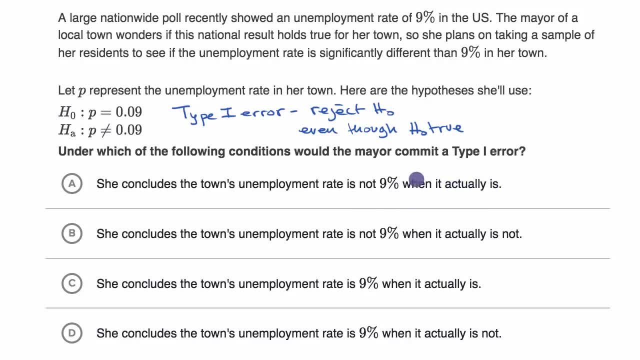 even though the null hypothesis is actually true, even though the unemployment rate actually is 9%. So I'm liking this choice. But let's read the other ones just to make sure. She concludes: the town's unemployment rate is not 9%, when it actually is not. 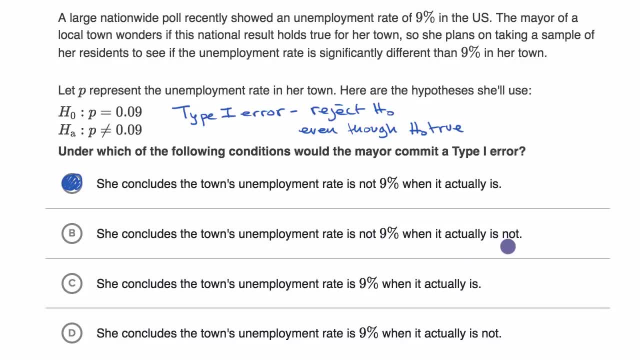 Well, this wouldn't be an error. If the null hypothesis isn't true, it's not a problem to reject it, So this one wouldn't be an error. She concludes the town's unemployment rate is 9%, when it actually is. 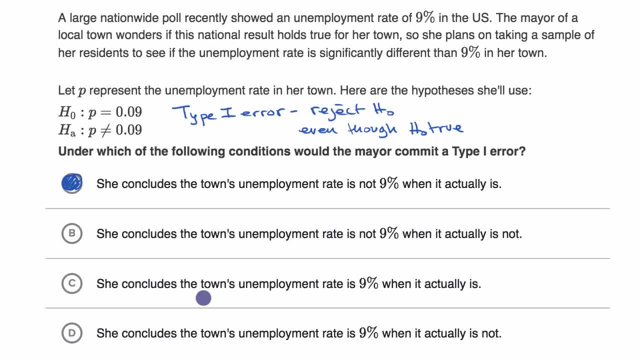 Well, once again, this would not be an error. This would be failing to reject the null hypothesis when the null hypothesis is actually true. not an error. Choice D: she concludes the town's unemployment rate is 9%, when it actually is not. 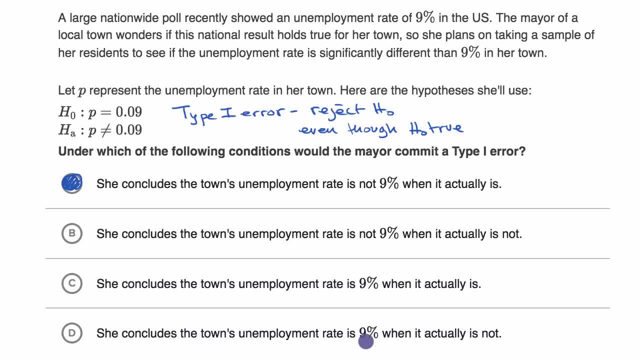 So this is a situation where she fails to reject the null hypothesis, even though the null hypothesis is not true. So this one right over here, this one would actually be. this is an error. This is an error. Well, this is a type two error. 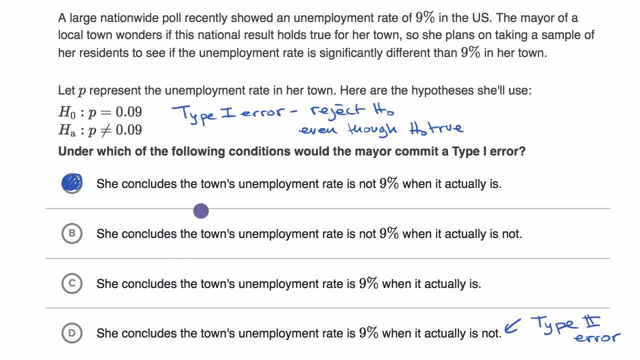 So one way to think about it. first you say, okay, am I making an error? Am I rejecting something that's true, or am I failing to reject something that's false? And the rejecting something that is true, that's type one. 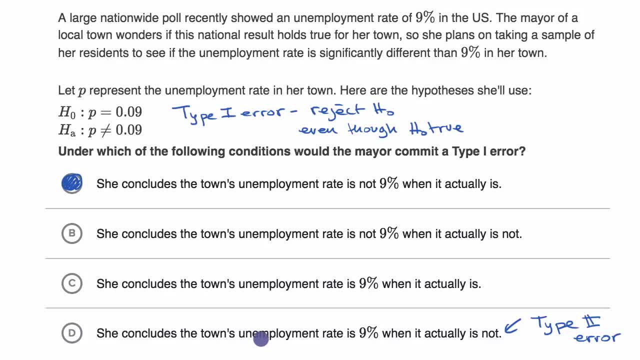 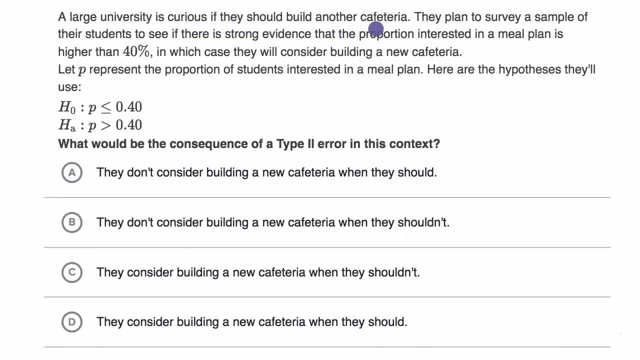 and failing to reject something that is false. that is type two. And so, with that in mind, let's do another example. A large university is curious if they should build another cafeteria. They plan to survey a sample of their students to see if there is strong evidence that the university is true. 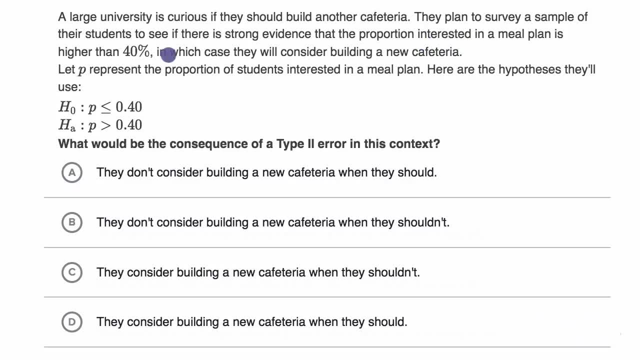 If there is strong evidence that the proportion interested in a meal plan is higher than 40%, in which case they will consider building a new cafeteria. Let P represent the proportion of students interested in a meal plan. Here are the hypotheses they'll use. 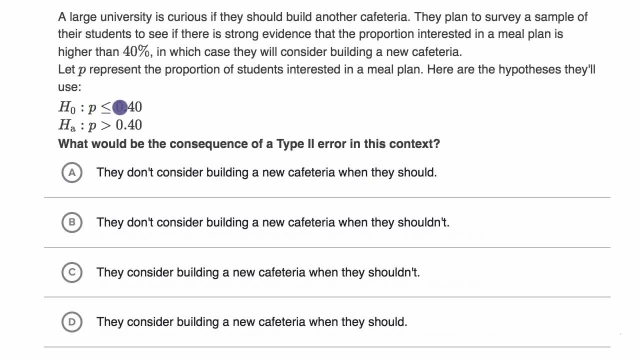 So the null hypothesis is that 40% or fewer of the students are interested in a meal plan, while the alternative hypothesis is that more than 40% are interested. What would be the consequence of a type two error in this context? So, once again, pause this video.